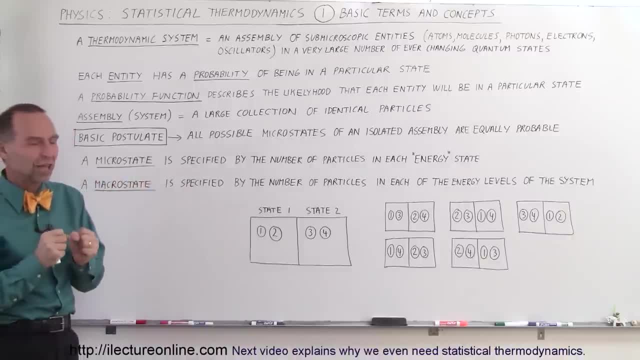 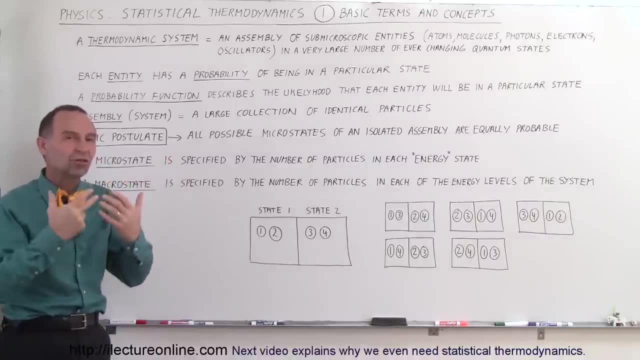 then we basically are dealing with a system. Now, to make it easier to understand, we'll first look at very small systems, because the numbers get to be really big. We'll look at very small systems and then, from understanding small systems, 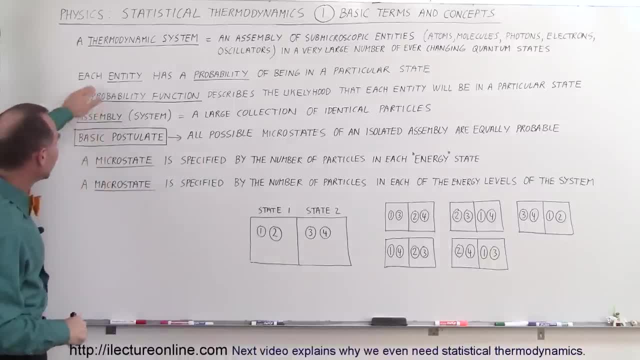 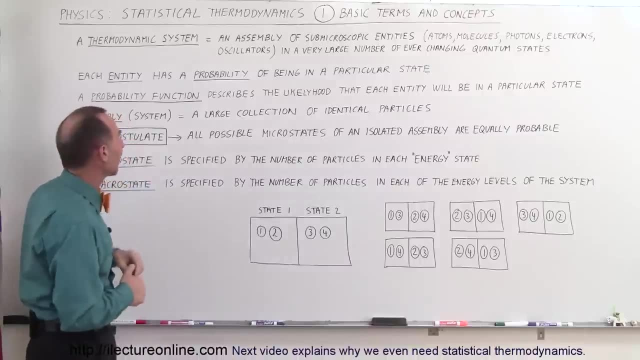 system. we'll build it up to larger systems, Each entity. so what do I mean by an entity? Well, an entity is just a small, either an atom, a molecule, a photon, electron, things like that- and each entity has a certain probability of being in a particular state. So usually, 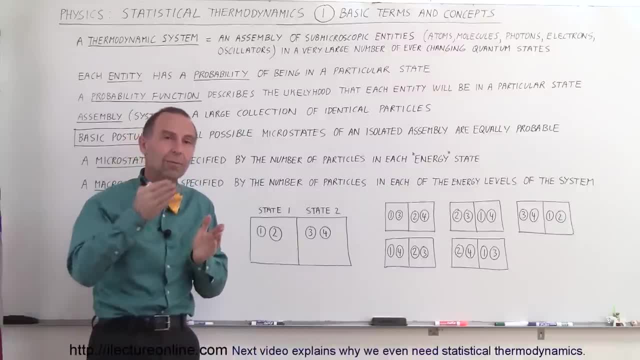 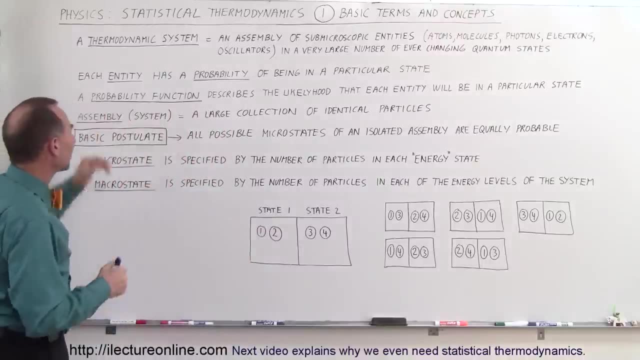 there's multiple states that they can be in, and so it has a probability. each entity has a probability in being one state or being in another state. Thirdly, we have to think about what we call the probability function. If you've ever taken a course in statistics, 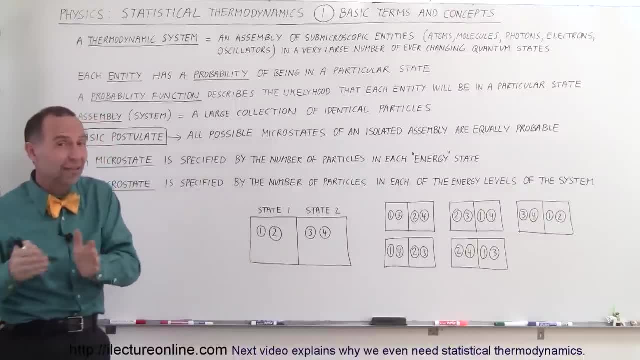 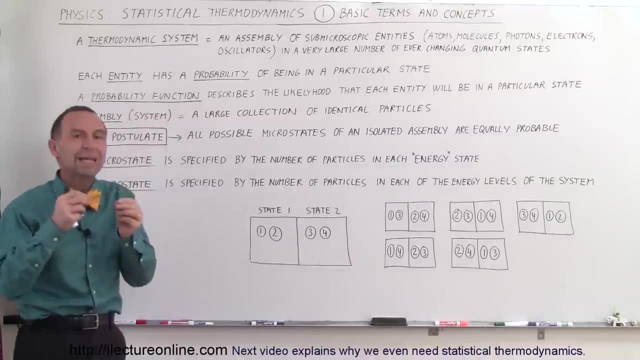 before then there's a lot of similarity between statistics and statistical thermodynamics. We use the very same principles and the big principle of that is what we call the probability of something being in a certain state, and to describe that. we'll describe that with. 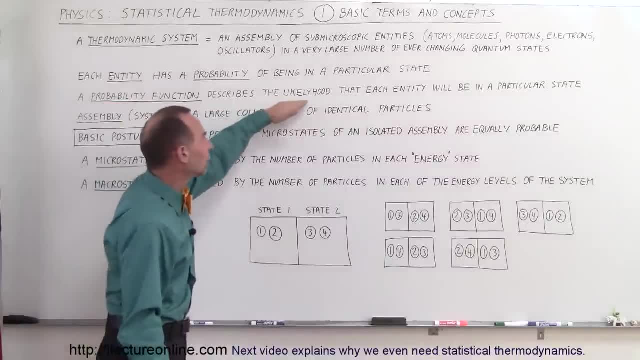 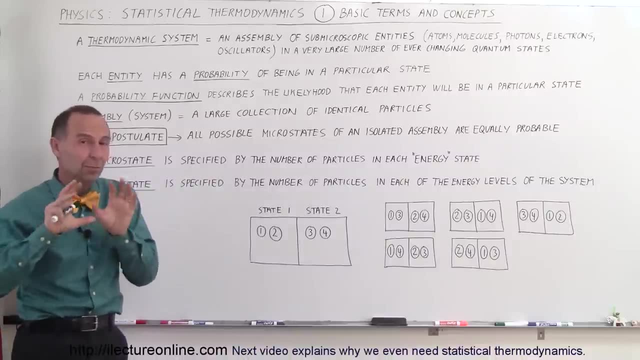 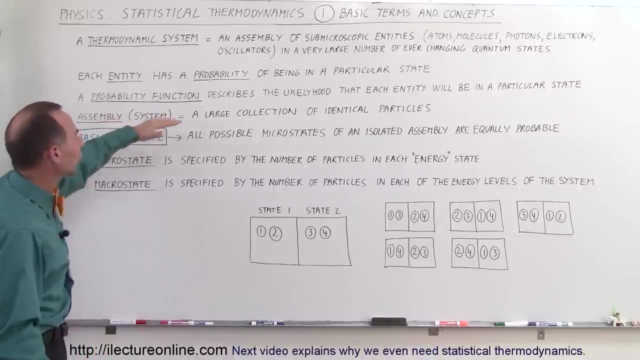 what we call a probability function. It describes the likelihood that each entity will be in a particular state. So you can imagine if there's many, many entities it can get very complicated, but we'll find a handle on it. We'll figure out how to understand that correctly. Again, the term assembly or system is a large 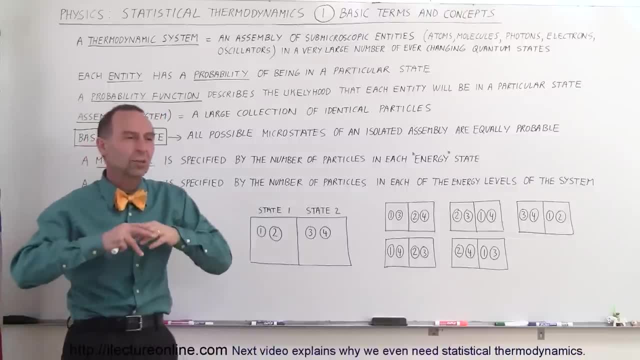 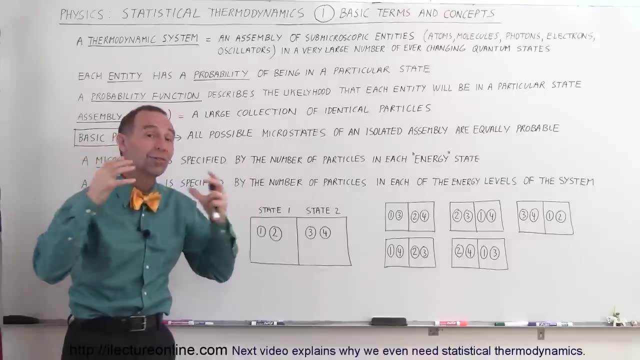 collection of identical particles. So typically we're not dealing with a mix of particles. we're dealing with a certain type of particles, a certain molecule, a certain atom, but it's always a great number of the same thing, so that they have the same properties, The basic. 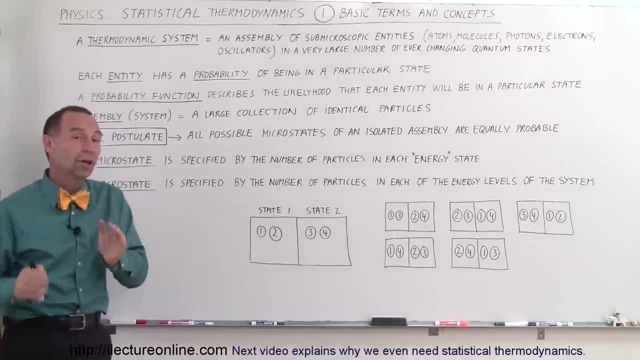 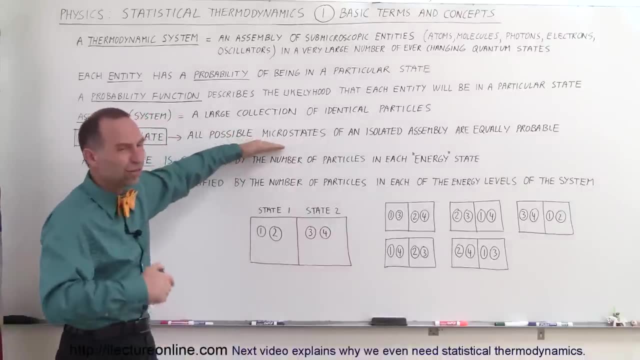 postulate. so when we're dealing with statistical thermodynamics, the basic postulate is that all possible microstates- and we'll define that in a second, but the basic postulate is that in just a moment, all possible, let's just say, states of an isolated assembly are. 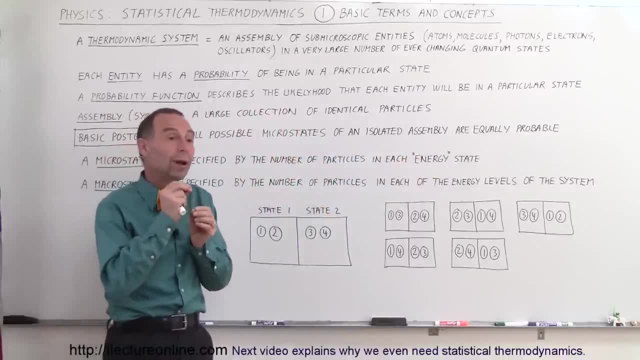 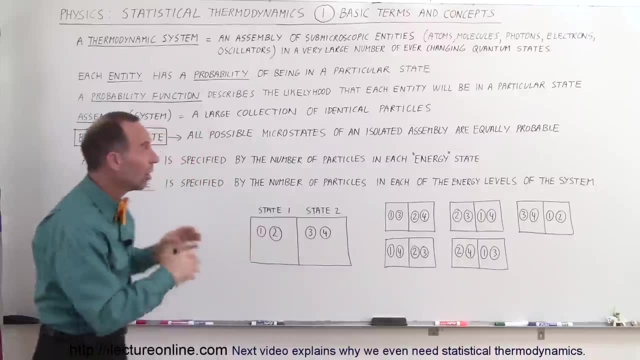 equally probable. So there's no case where it's more probable to be in state A than to be in state B. They have equal probability and that is very important. That is the postulate of statistical thermodynamics, so we usually assume that to be the case. 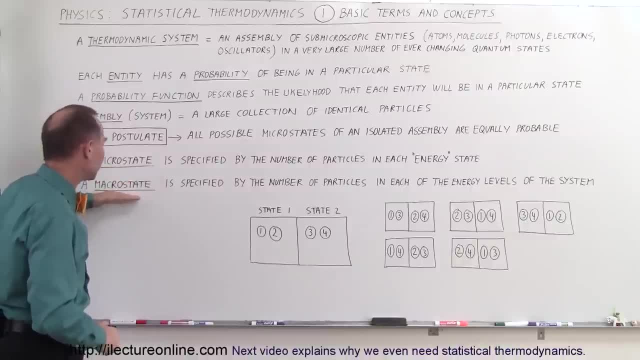 Now we have the difference between what we call a microstate and a macrostate, and that's very difficult to define in words. So we'll give it a try, but then I have to give it a try. I have something here on the board that will help us understand the difference between. 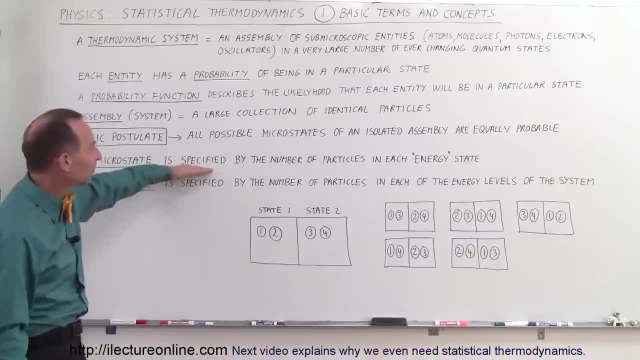 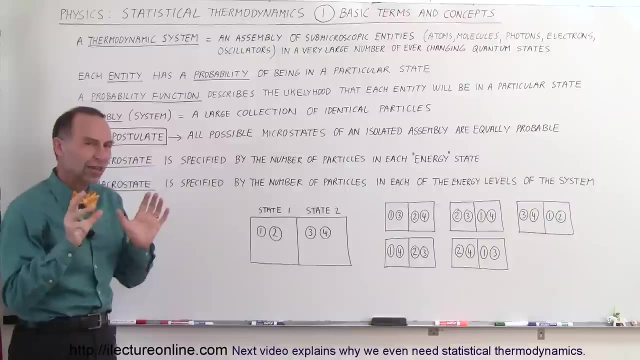 them. So a microstate is specified by the number of particles in each energy state. So, again, a microstate is specified by the number of particles in each energy state. It's actually a little bit different from that as well, so let's hang out to that definition. 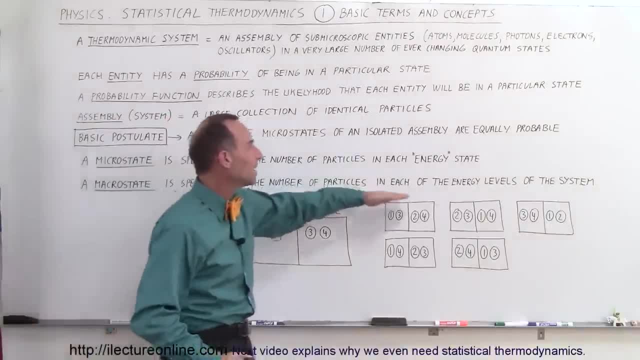 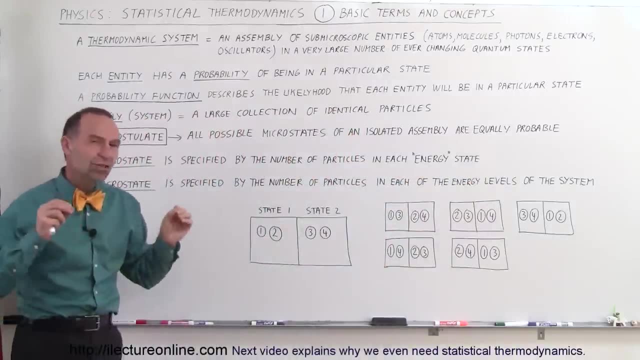 And a microstate is specified by the number of particles in each of the energy levels of the system. Now, what do we mean by that? Okay, much in nature is driven by energy, and down at the quantum mechanical level, we always deal with energy states. When we look at electrons inside an atom, they can 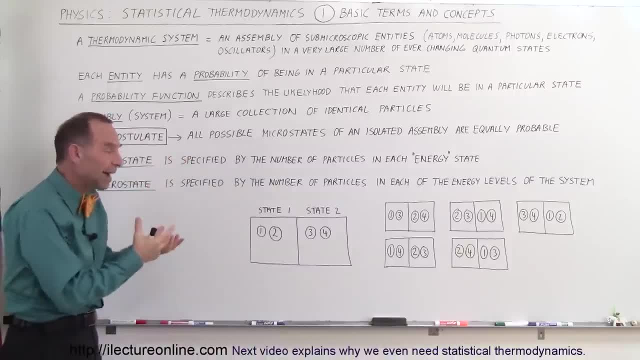 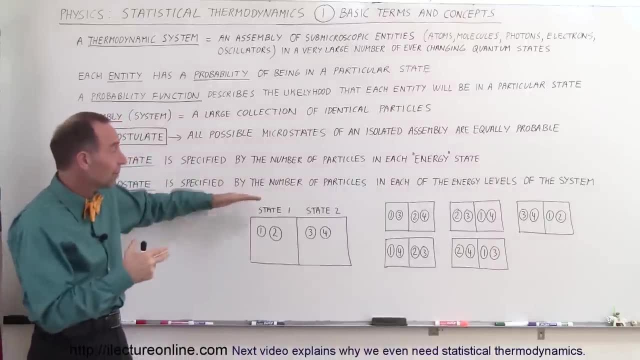 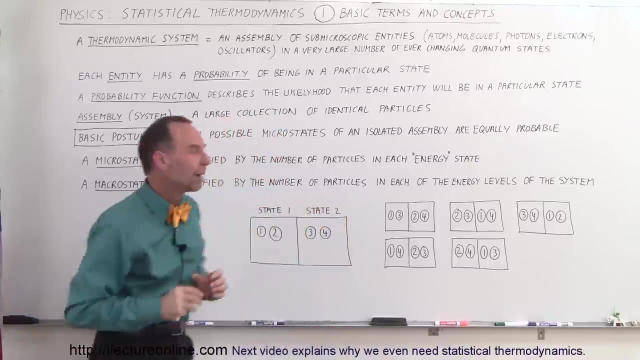 be at various energy levels. So therefore, we can then define the microstate by knowing how many of each item of the assembly, how many of each of the particles of the assembly, are in each of the different energy levels. That will then define a microstate. 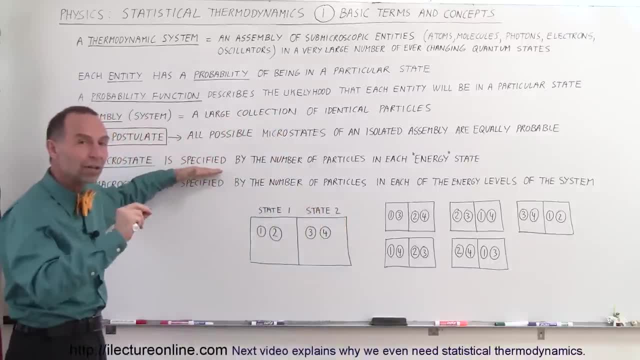 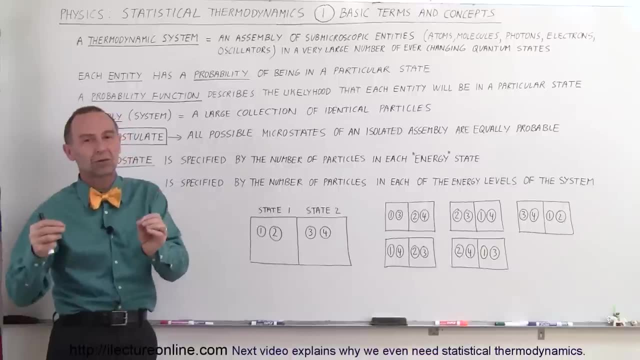 And then we can go look at each of the particles and see which particle is in which state. and that defines the microstate, And usually there's a number of microstates for each microstate. So a microstate is usually a sub-portion of a microstate. 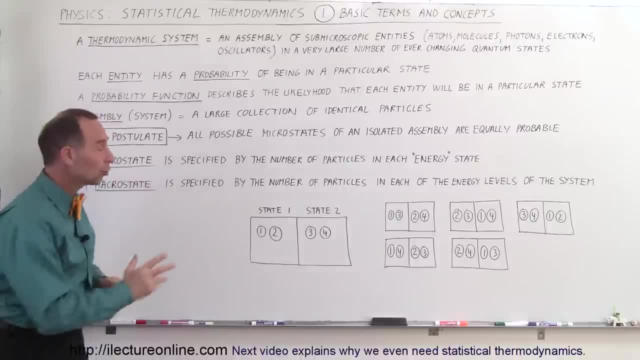 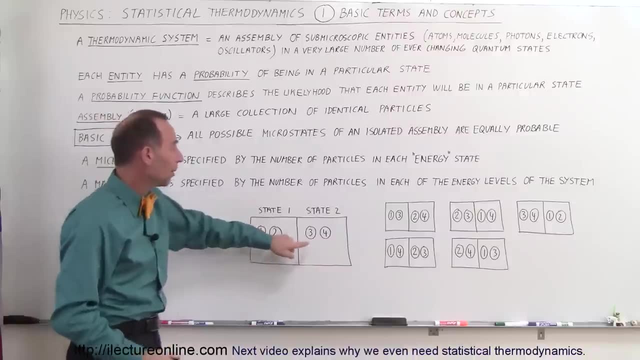 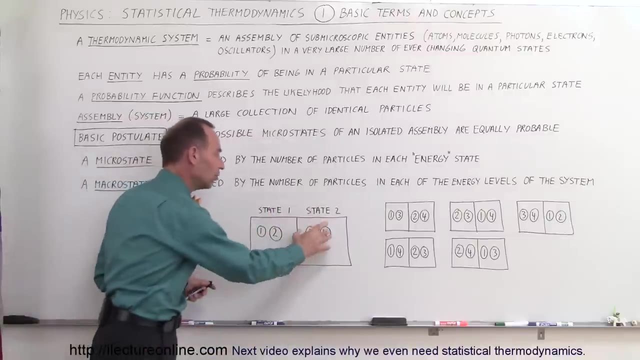 Alright, now let's try to define it graphically. Let's say there are two states and there are four particles. In this particular case, we have particle one and two in state one and particle three and four in state two. So having two particles in state one and having two particles in state two out of 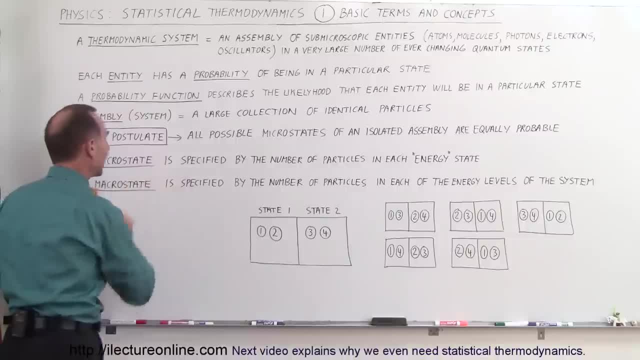 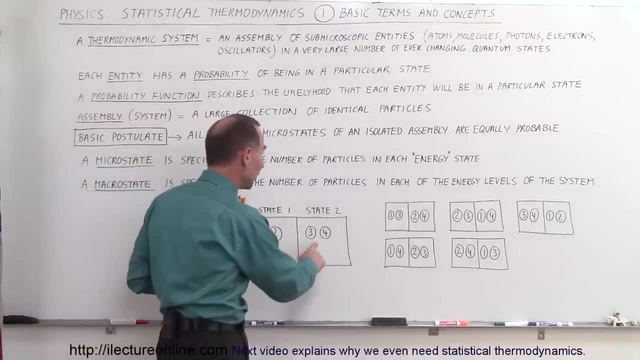 a total of four particles will be defined as a microstate. But it turns out that we can actually interchange those particles. For example, we can move particle two to state two and particle three to state one. Now we have a different arrangement. 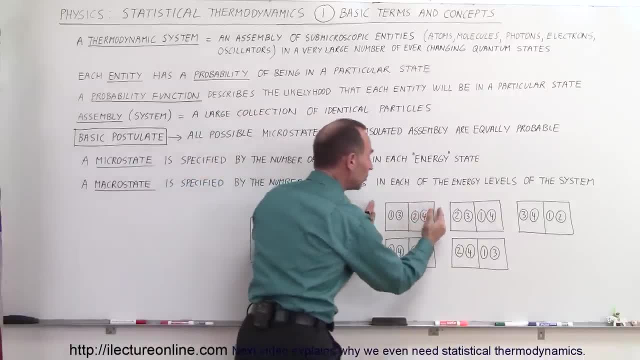 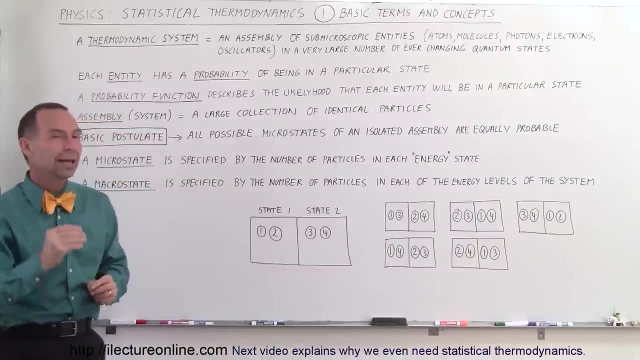 So this would be called a microstate. This is another microstate, but notice, in both cases we still have two particles and two particles in each state, two in state one and two in state two. So this is the same microstate but a different microstate.